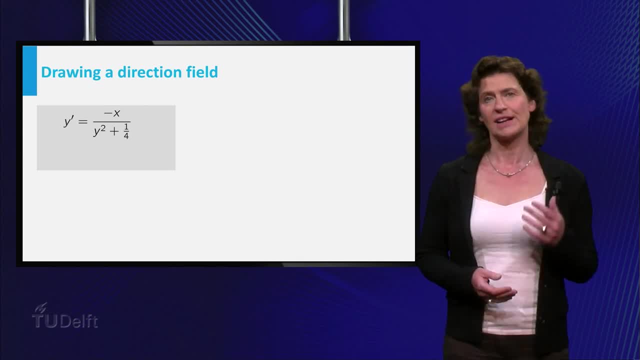 Solving this differential equation means that you want to find all functions, y depending on x, that satisfy the equation. Finding solutions to differential equations in general is quite hard. In this course you will learn how to solve certain classes of differential equations. But as long as you don't know how to do this, you can draw a direction field to get. 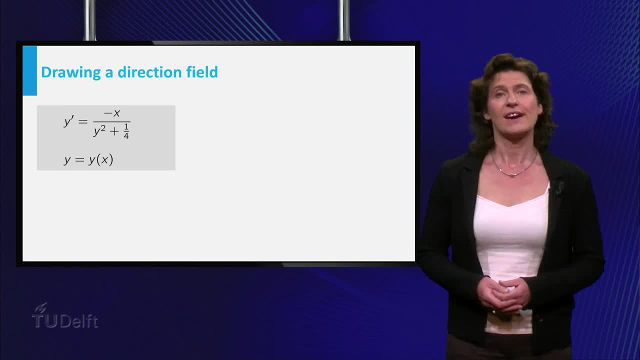 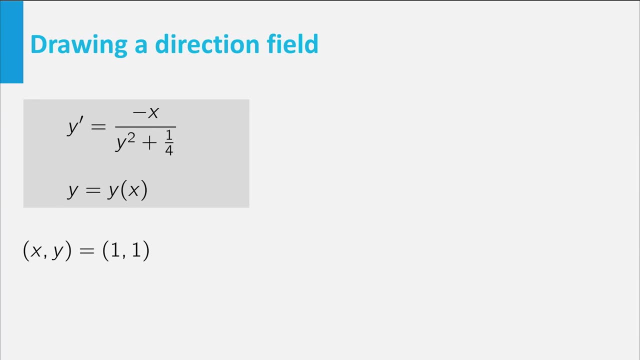 an idea of what the solutions look like, Let's find the direction field for the differential equation you see here. Now suppose the graph of a solution of this equation passes through the point. This means, of course, that for x equal to 1, the corresponding value of y of the solution. 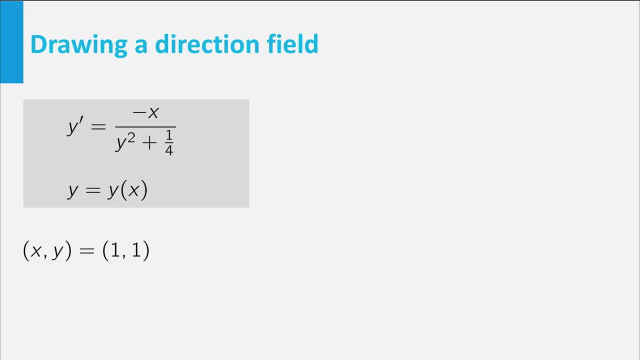 is equal to 1.. From the differential equation it follows that the derivative of the solution in 1 equals minus 1 divided by 5. fourth, which is minus 4. fifth, What does this mean? It means that the tangent line at the graph of the solution in the point has slope. 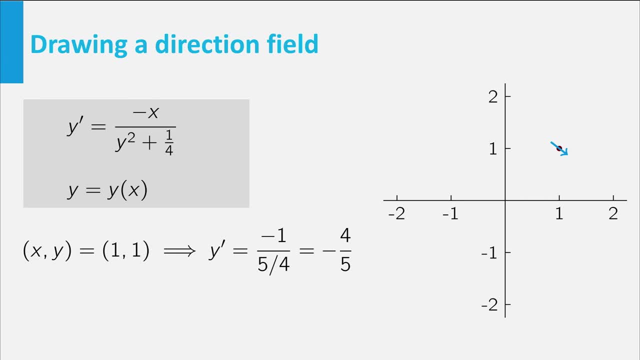 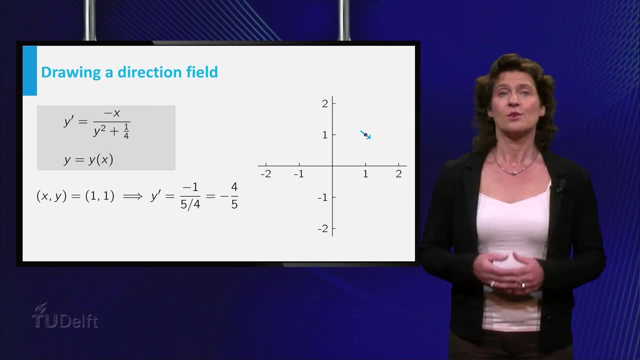 minus 4 over 5.. Here you see a small part of this tangent. So, without having solved the differential equation, without knowing the explicit formula for the solution of the differential equation, you found the slope of the graph of the solution at x equals 1.. 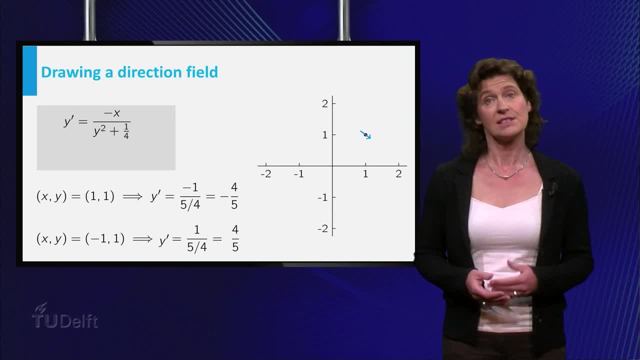 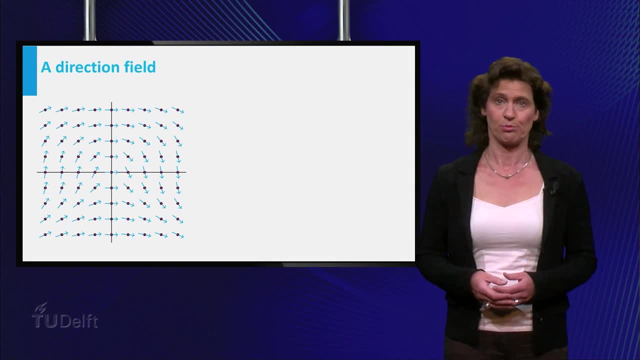 For the point, the slope of the tangent is equal to plus 4 over 5.. Here it is. You can do this for many other points and get this beautiful picture. This is called the direction field. What do you see in this picture? 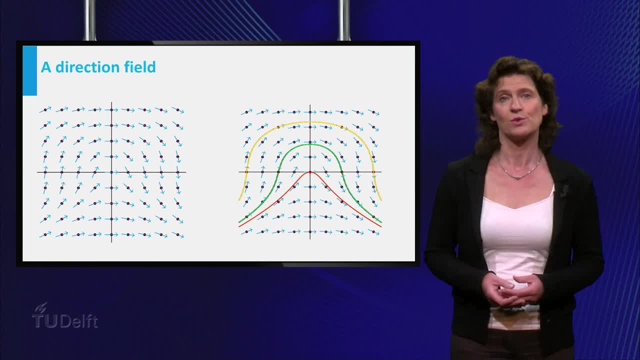 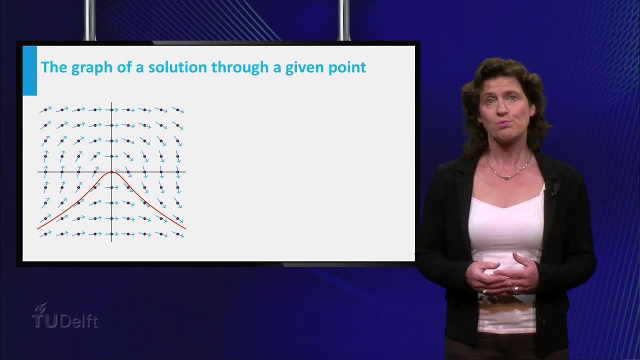 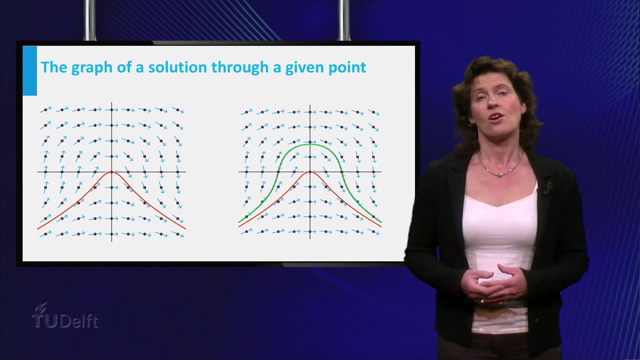 Well, you can draw the graph of a solution with given starting points by following the direction field like this. So the graph corresponding to the solution of the differential equation which passes through the origin is the orange one. The solution which passes through the point has the green graph. 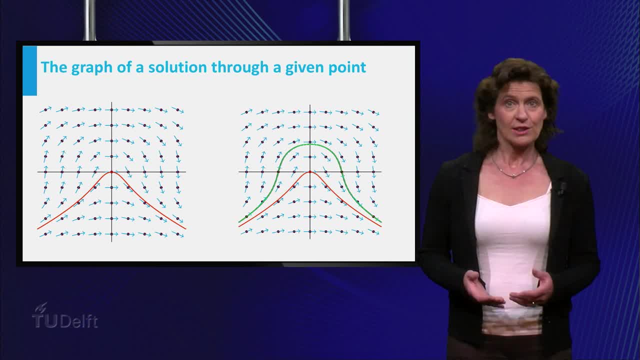 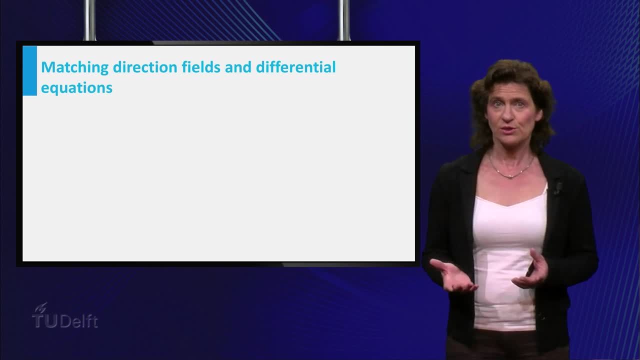 Obviously, drawing a direction field by hand is tedious. Luckily, there is software that can do the job for you. Now let's see if we can identify two direction fields corresponding to two different differential equations. Here are the equations: y' is equal to x times 2..